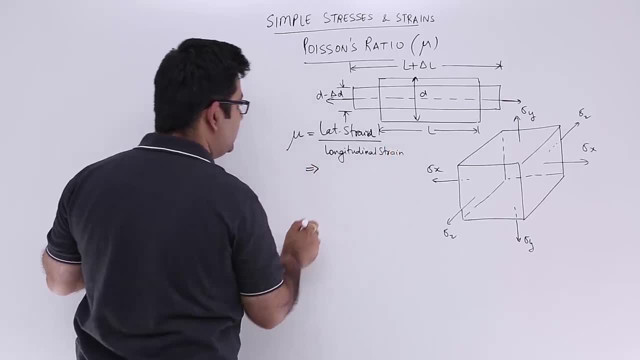 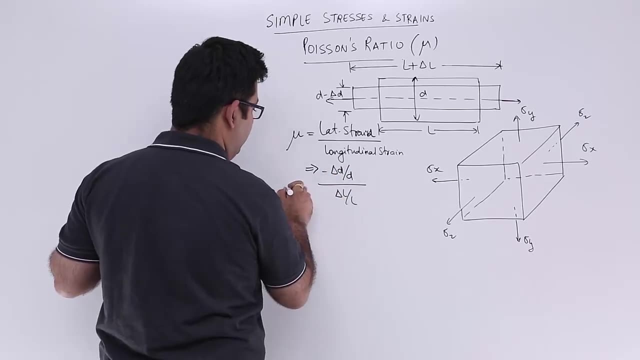 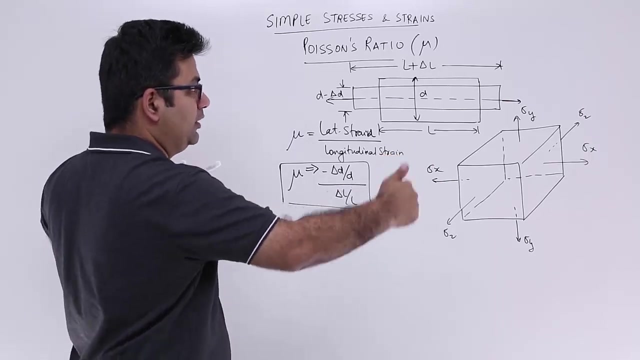 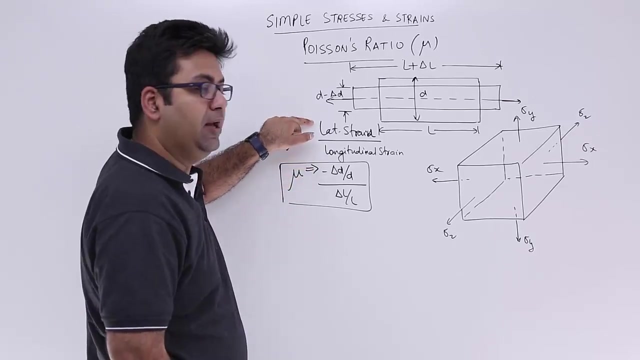 Okay, So this means this is equal to minus delta D upon D upon delta L upon L. So this is what we understand mathematically by mu. If you compress it upon compression, your longitudinal strain will be a negative value, but your lateral strain will be a positive value, So you will again have a negative in this fraction. Okay, 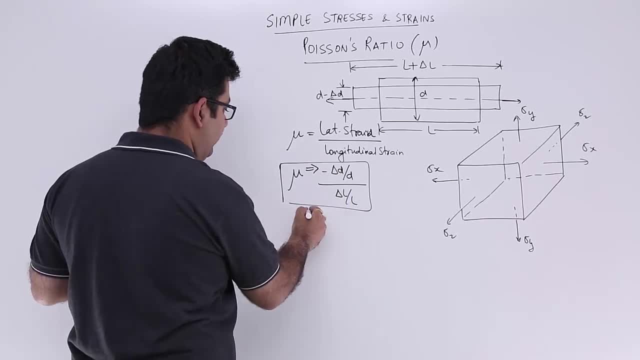 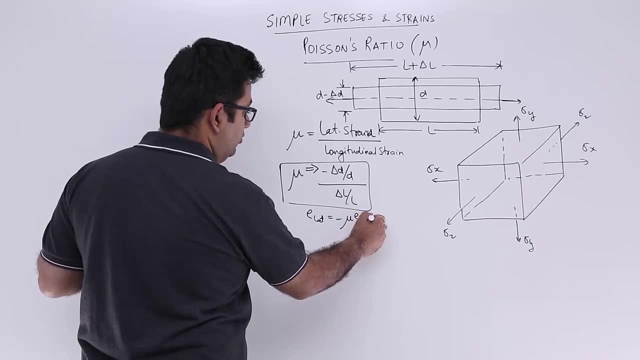 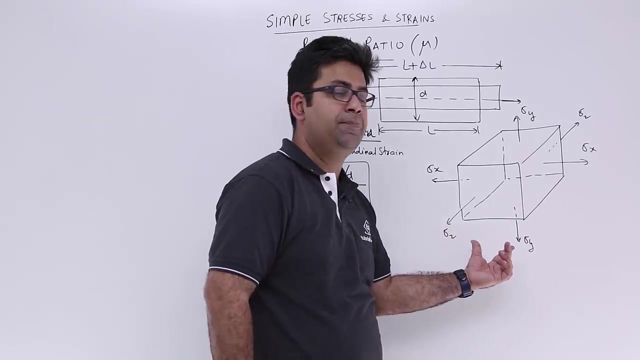 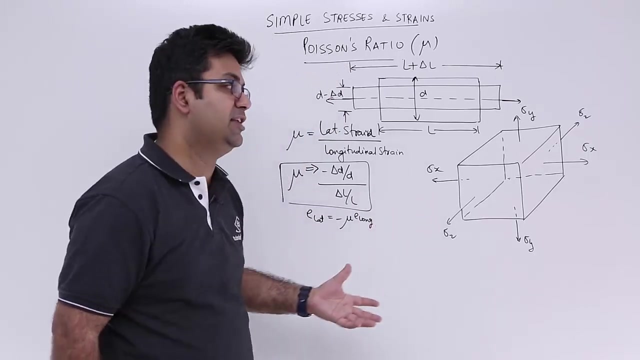 Now this means that the lateral strain, which is e lateral, this is equal to u mu by e longitudinalурm. So make use of this concept. You are understanding this thing, which is a, I would say, multi axial stressing of a body. We are trying to strain the body in multiple axes. This is uniaxial straining. 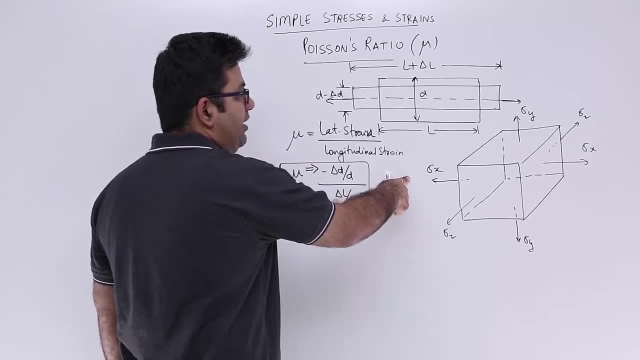 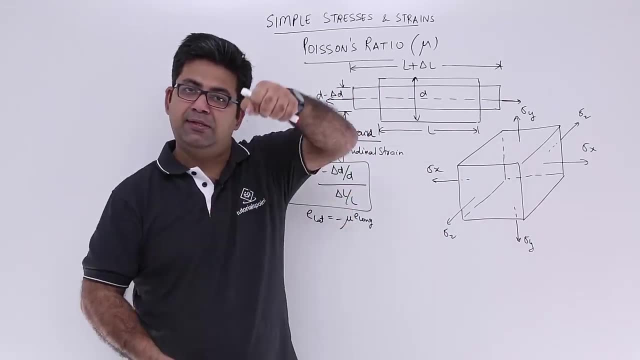 of the body. Now, in this, what is happening? Now, in this, what is happening, you have a stress value in the x direction, in the y direction and in the z direction, so you are pulling the body like this, like this and like this. okay, so, due to sigma x, 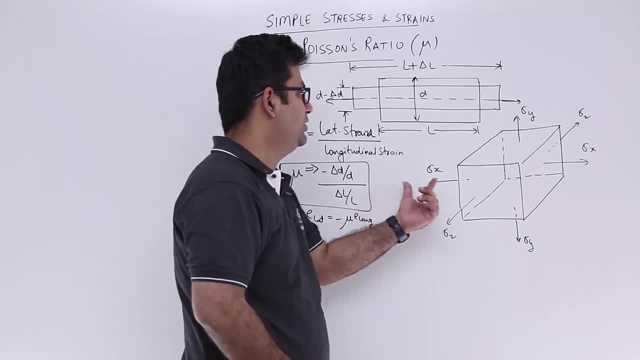 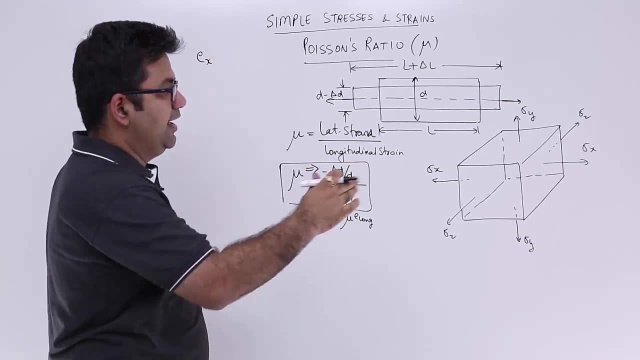 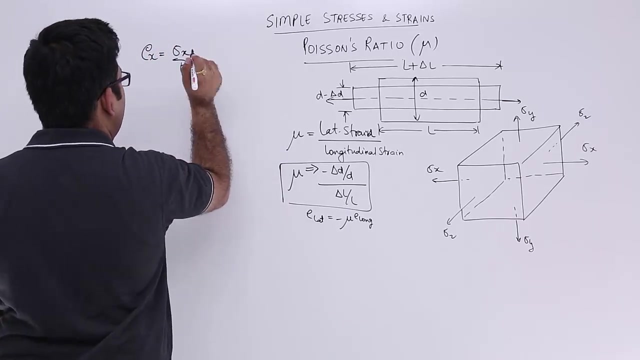 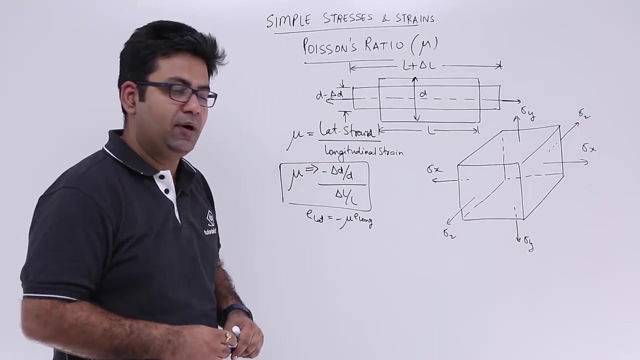 there will be some elongation in the direction x. so let us say that is ex, that is the straining in the x direction. okay, let me write it down again. so this is ex, which is sigma x upon e. but when you pull the body in the direction of x, what happens to the dimension y and dimension? 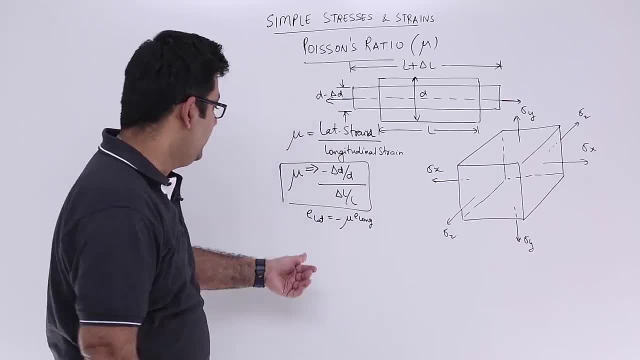 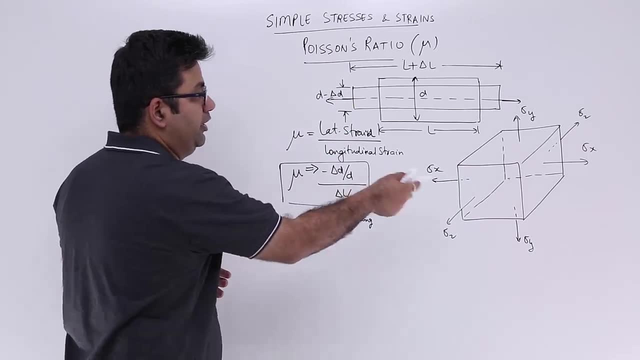 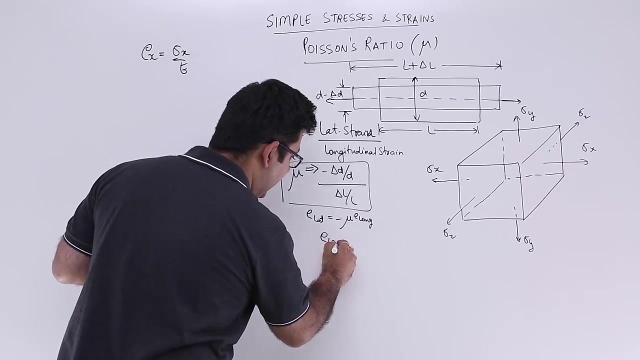 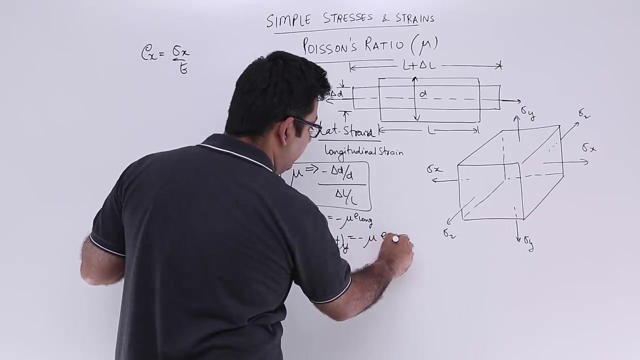 z, they get contracted. so there is some lateral straining in the direction of y and in the direction of z due to a longitudinal straining. So the lateral straining in x, so the lateral strain in y, if I write it down like this, the lateral strain in y, this is equal to minus mu- into longitudinal strain in the direction. 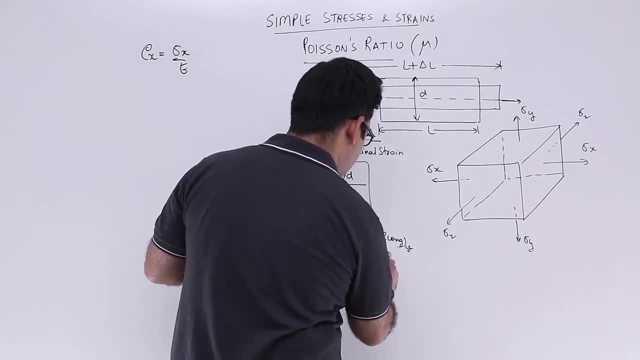 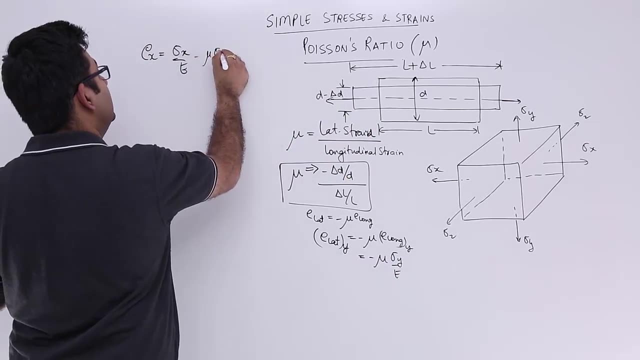 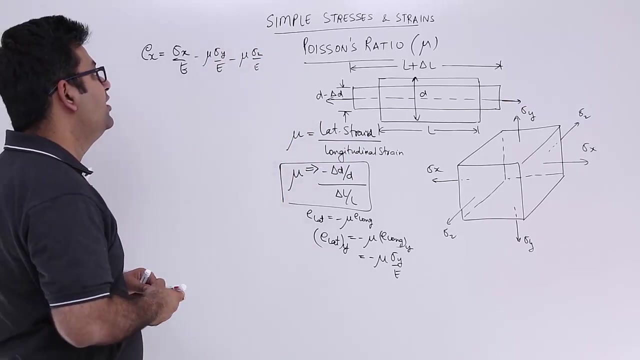 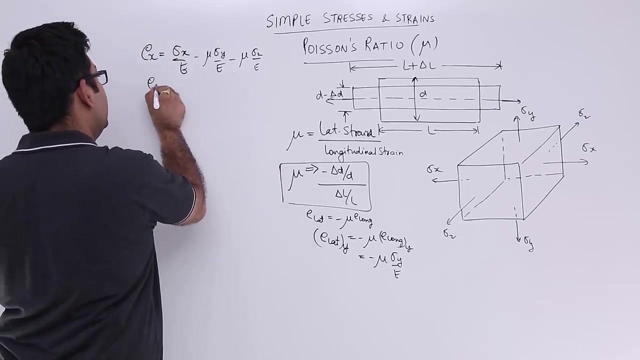 of y, which is equal to minus mu sigma y by e. this would be minus mu sigma y by e. similarly in the direction of z. So in the direction of z axis, you will have again a lateral strain of minus mu sigma z by e. so this was for x axis. what about for y axis? so for y axis again, the longitudinal. 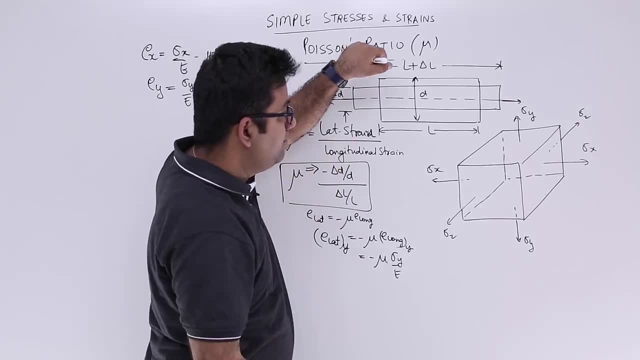 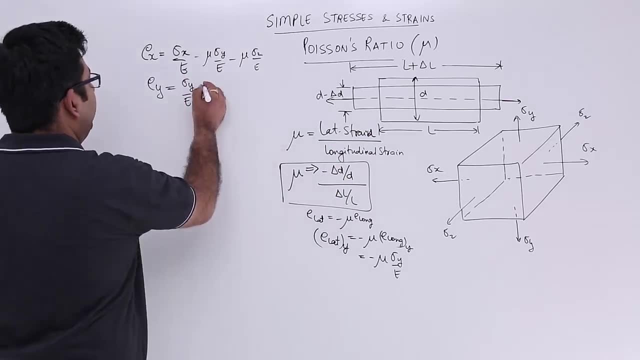 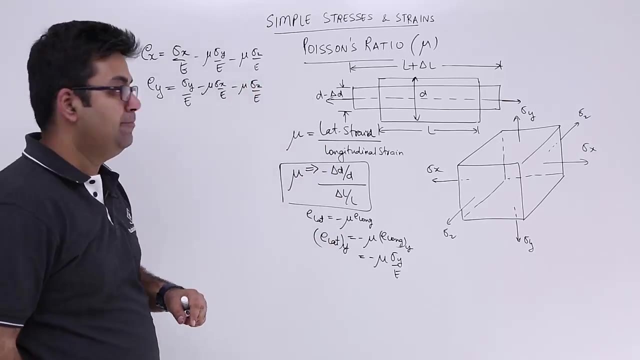 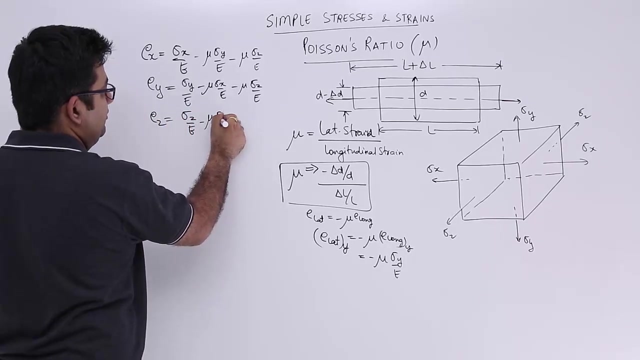 strain would be sigma y by e, but due to the pulling in the y direction you have some lateral contraction in direction x and in direction z, so that would be compensated by this value minus. Okay. similarly, if you come to ez, you get sigma z upon e minus mu, sigma x upon e minus. 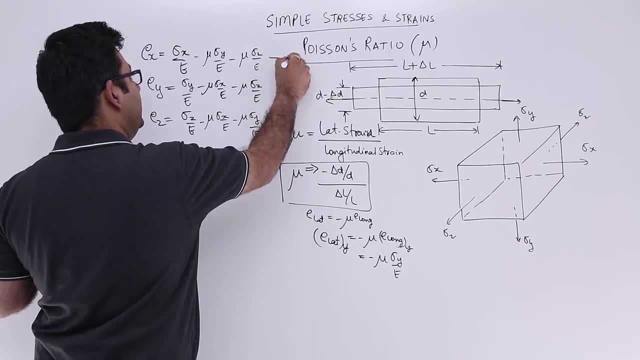 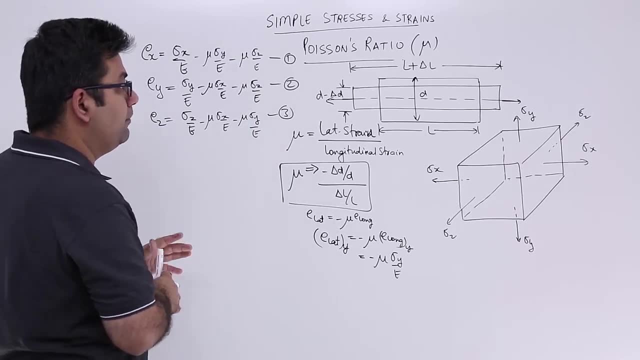 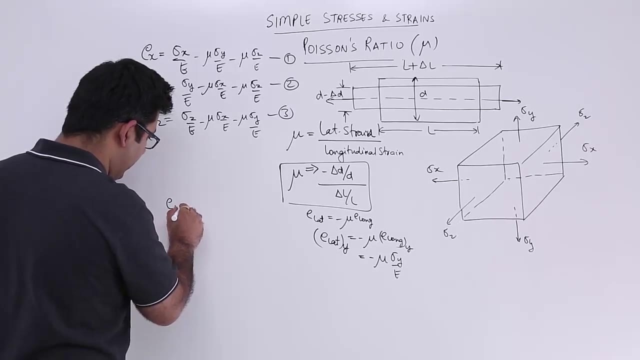 mu, sigma y upon e. so this is, let us say, equation 1, equation 2, equation 3, so you have strains being produced in all the three directions. if you have to find out the value of the total strain, So you will have to add all these three up. so you will be adding 1 by e, sigma x plus. 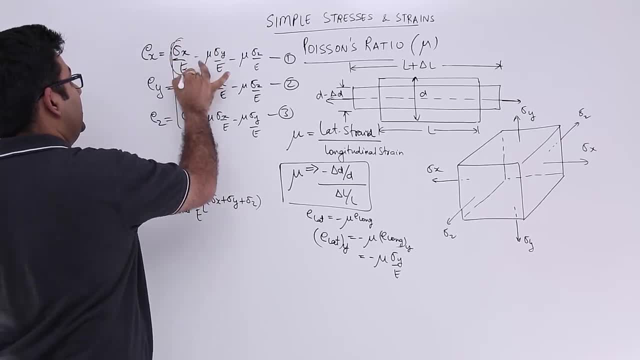 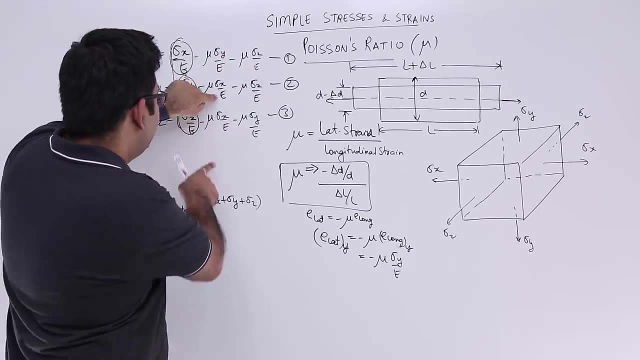 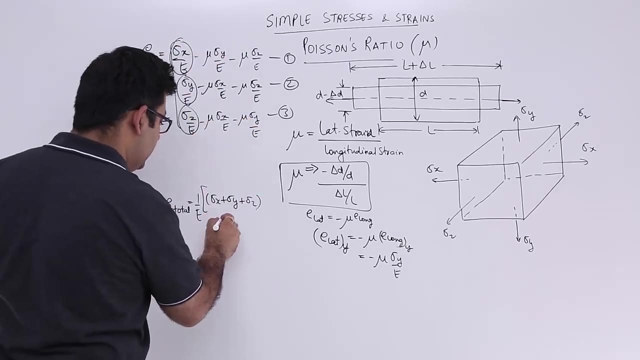 sigma y plus sigma z. that is this part, this part, this part. now, if you start adding these six terms, you have twice the sigma x, you have twice the sigma y and you have twice the sigma z. So it will be minus 2 mu sigma x.